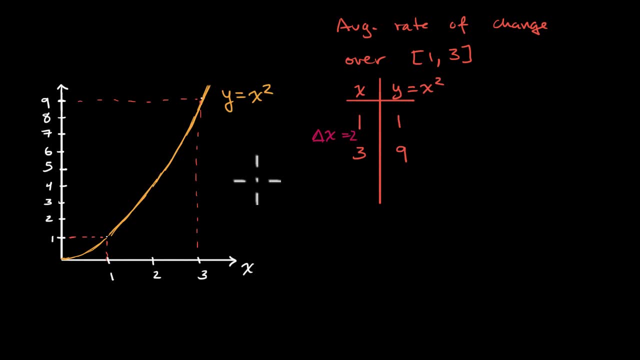 Well, what's our change in y over the same interval? Our change in y is equal to when x went, increased by two, from one to three. y increases by eight, So it's gonna be a positive eight. So what is our average rate of change? 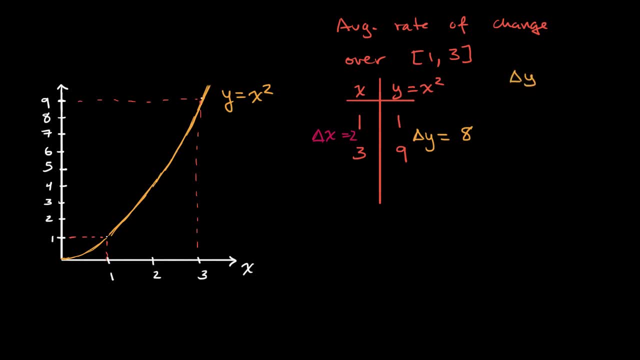 Well, it's gonna be our change in y over our change in x, which is equal to eight, over two, which is equal to four. So that would be our average rate of change Over that interval. on average, every time x increases by one, y is increasing by four. 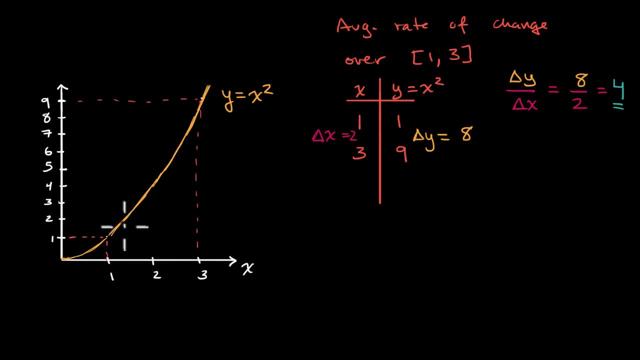 And how did we calculate that? We looked at our change in x. Let me draw that here. We looked at our change in x and we looked at our change in y, which would be this right over here, And we calculated change in y over change of x. 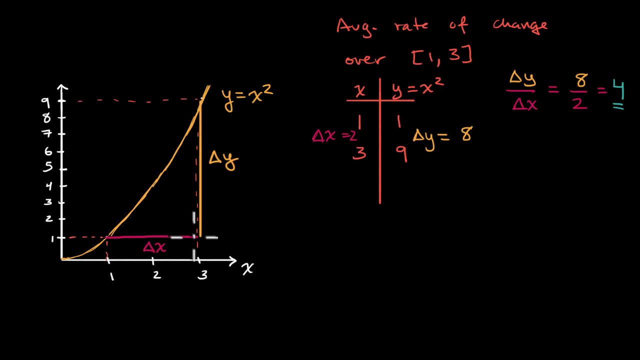 for average rate of change. Now, this might be looking fairly familiar to you, because you're used to thinking about change in y over change in x as the slope of a line connecting two points, And that's indeed what we did calculate. If you were to draw a secant line between these two points, 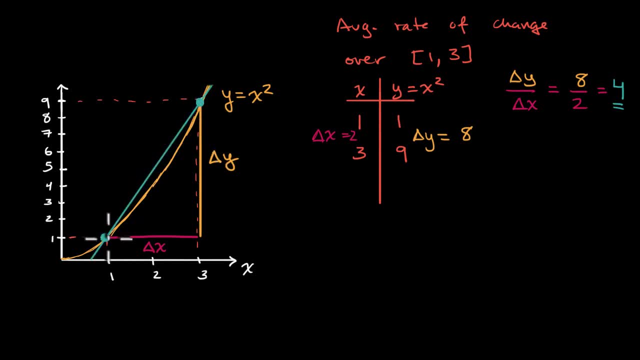 we essentially just calculated the slope of that secant line And so the average rate of change between two points. that is the same thing as the slope of the secant line, And by looking at the secant line in comparison to the curve over that interval. 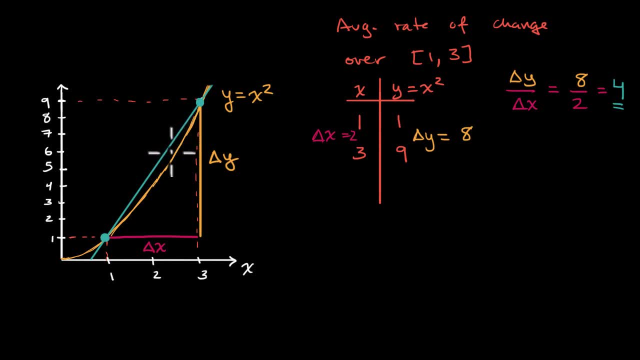 it hopefully gives you a visual intuition for what even average rate of change is. So let's look at the slope of the secant line and see what average rate of change means, Because in the beginning part of the interval you see that the secant line is actually increasing. 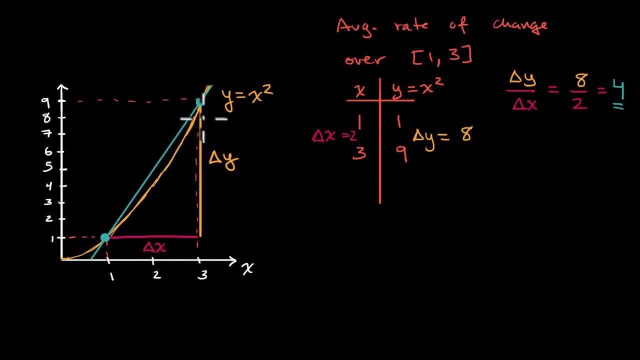 at a faster rate, but then, as we get closer to three, it looks like our yellow curve is increasing at a faster rate than the secant line, and then they eventually catch up, And so that's why the slope of the secant line. 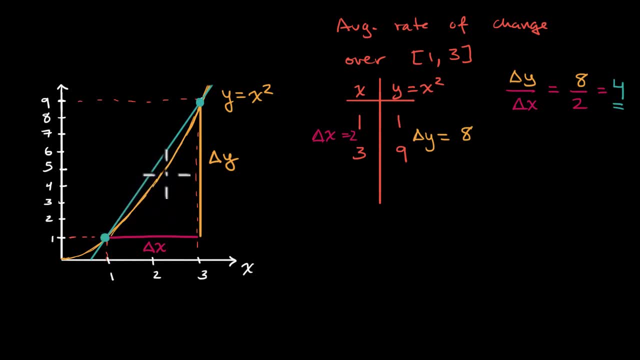 is the average rate of change. Is it the exact rate of change at every point? Absolutely not. The curve's rate of change is constantly changing. It's at a slower rate of change, at a higher rate as we get closer and closer to three.